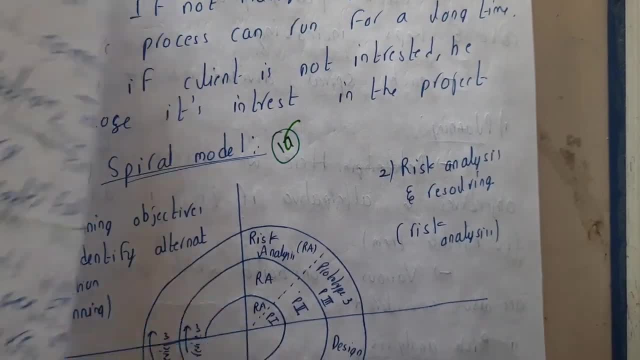 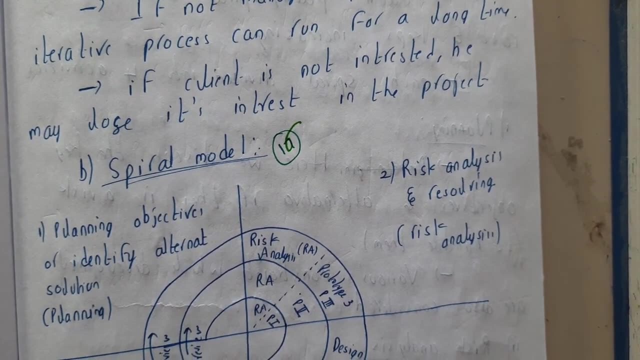 So basically, here in this all steps, we never, we are never calculating the risk factor right? So if you recall, even in the waterfall model in SDLC we are not calculating about risk. So basically, this spiral model is used for the projects which are intended to go to risks. 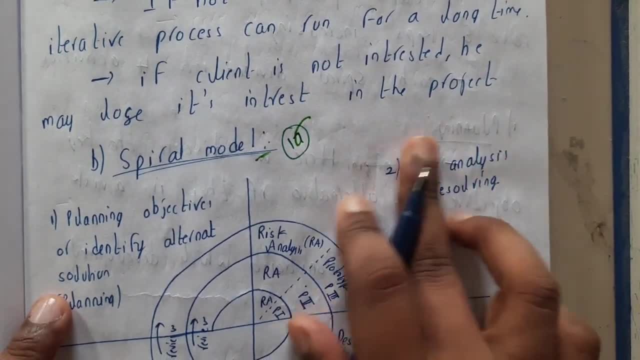 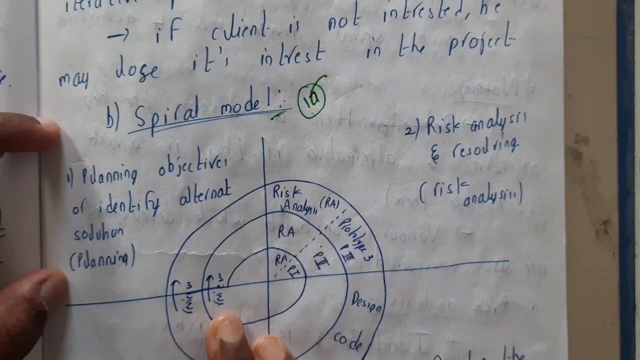 They will be using this spiral model, guys. So in spiral model, you are having a particular phase for risk analysis and resolving the risks, guys, Okay, Okay. So let us go through the first step. There are four steps, guys, For this diagram is really simple: Just draw an axis and you just start drawing a spiral. 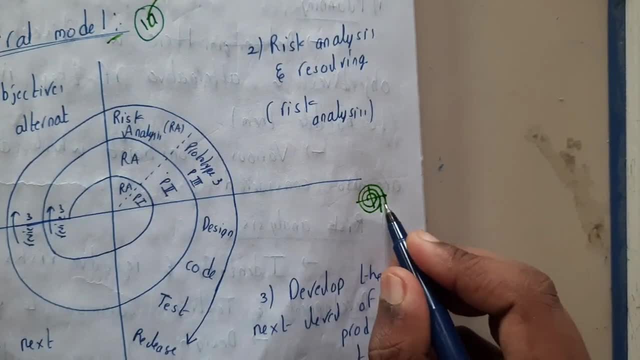 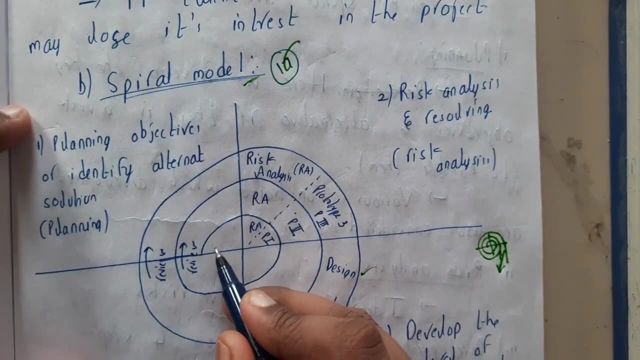 Okay. So at the end from here, you will be getting your output. That is nothing but designing, coding, testing, and release will be in this way. Okay, Similarly, you will be starting from interior guys. So the first stage is nothing but planning objectives or identifying alternate solutions. 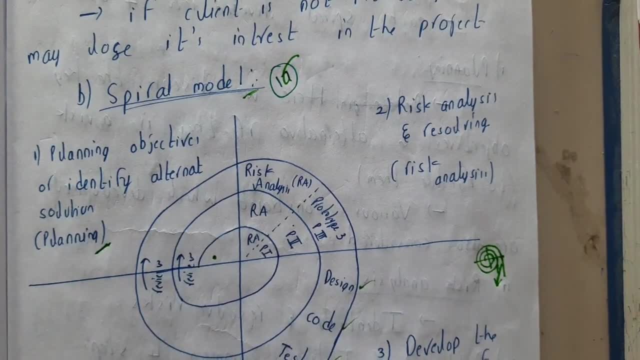 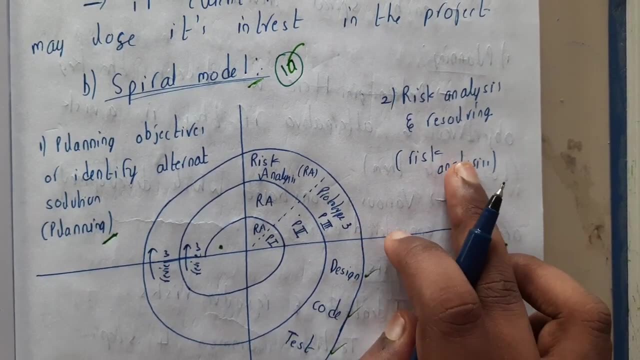 That is nothing, but, in simple words, we will be playing. we will be saying it as planning- Okay. The second phase is nothing but risk analysis and resolving. So, in common words, you will be saying it as risk analysis phase, Okay. So remember that. 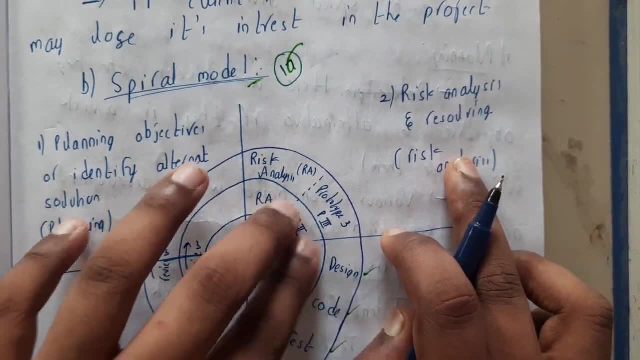 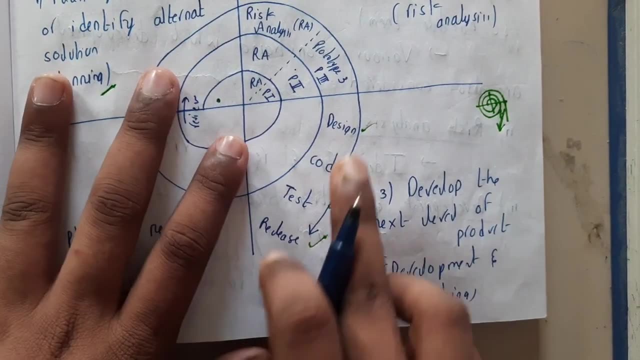 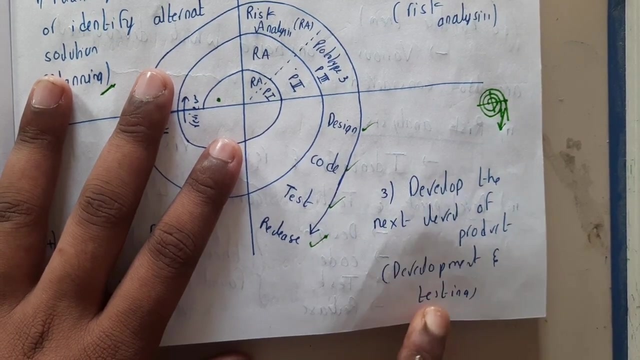 In risk analysis phase only. we will be doing risk analysis as well as prototyping. You can say that prototyping is the third phase, but they will be doing in the same phase only guys. Okay. Similarly, in the phase three, that is nothing but a deployment or development. the develop the next level of product. that is nothing but development and testing. 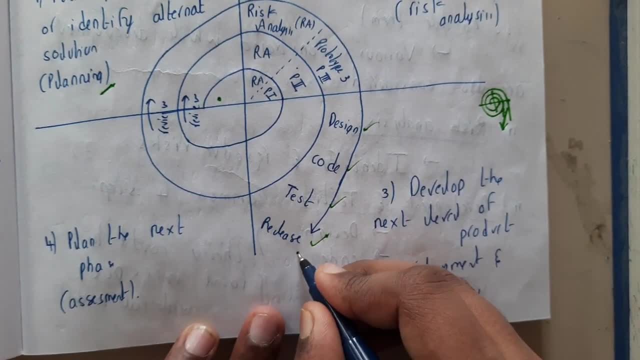 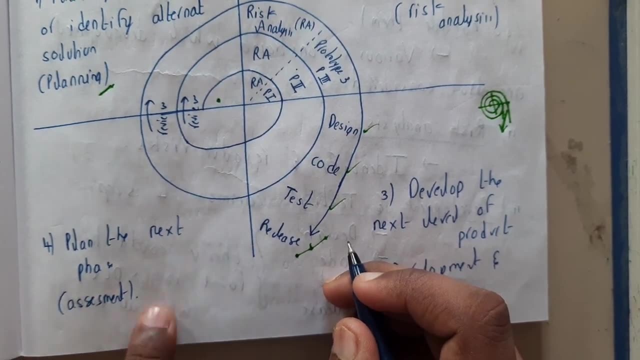 So here only you will be doing testing and everything else, And here only you will be releasing it. Okay, So the next phase is nothing but assessment. So you released the product right. So you'll be getting multiple reviews, So you'll be assessing the product. 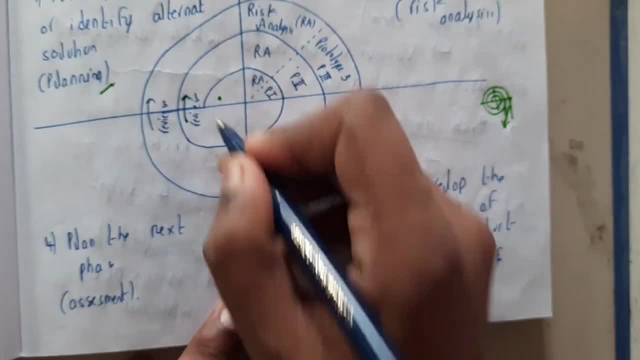 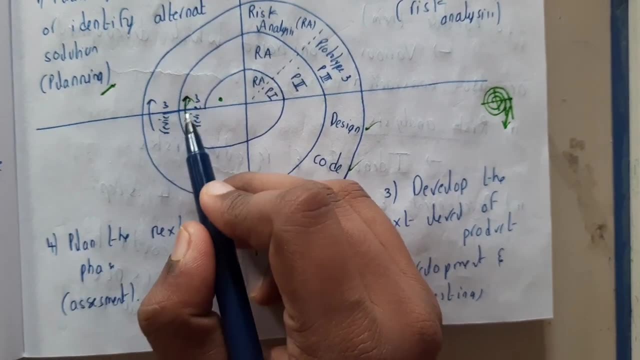 So you'll be getting multiple reviews, So you'll be assessing them and you'll be informing about those resolutions, or the solutions, or the bugs and everything you'll be informing again to the, again to planning. So again they will be planned for it and the process continues. 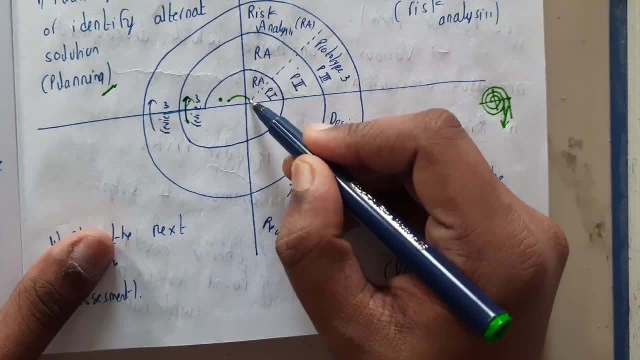 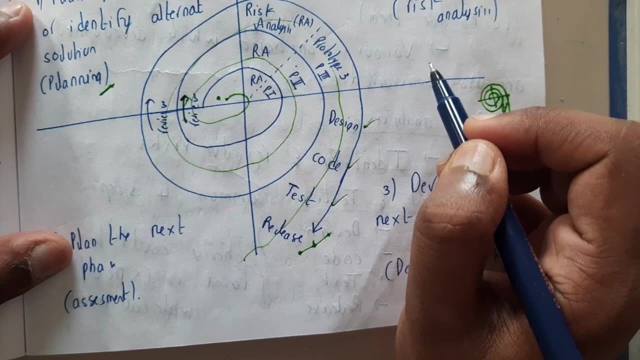 So if you observe, here the process starts, here It goes in this way, It goes exactly in the form of a spiral. So that is the reason why this model is called as spiral model. Okay, Guys, as usual, most of the theoretical part about planning and everything planning. 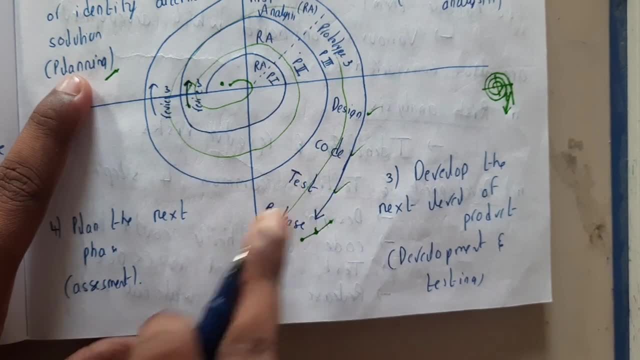 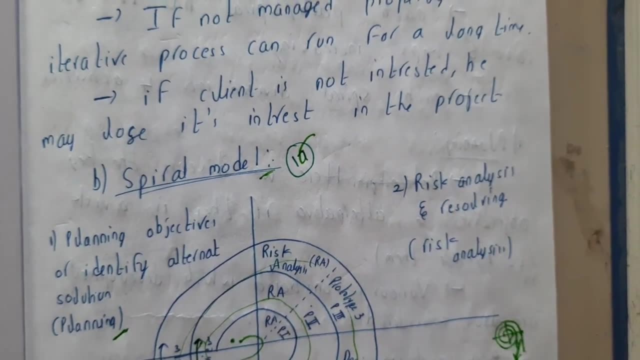 And prototyping and developing, testing, coding every theory. we have already discussed about the theory concepts of that, So I'll be just giving you an introduction and we'll be discussing about risk guys, because we didn't discuss about risk, Right? Okay? 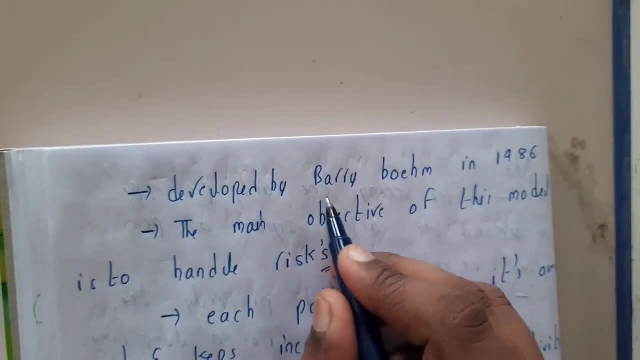 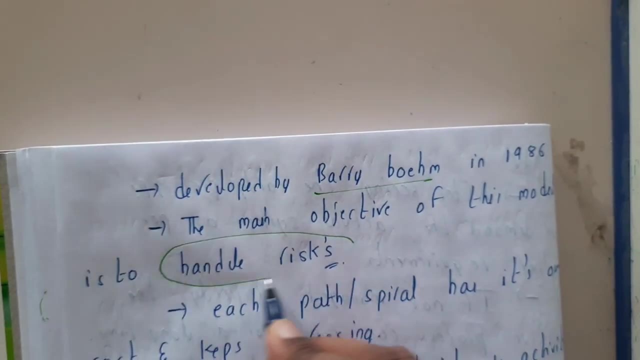 So it was developed by Barry Bohem in 1986.. Okay, The main objective of this module is to handle this. I told you right. So the main objective of this model is to handle risk. So each path or spiral has its own concept. 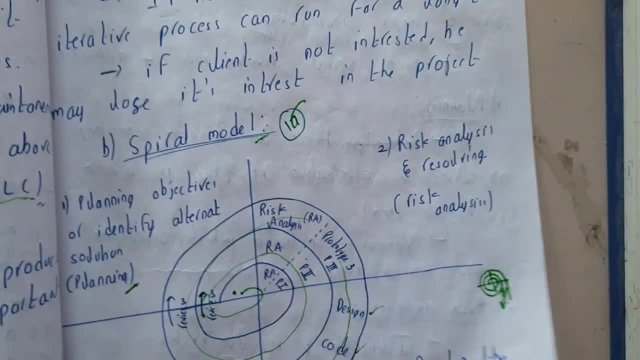 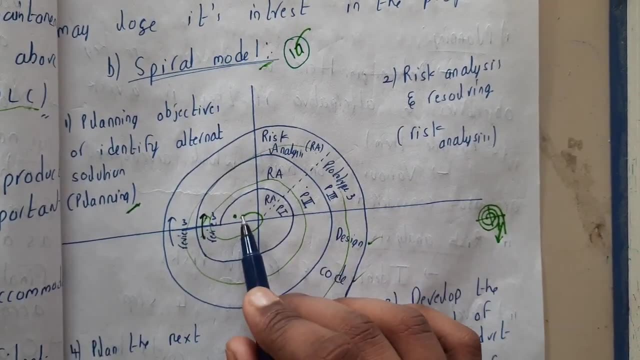 It has its own cost and it keeps increasing. So we already learned about incremental model and everything right. So this is almost like an incremental model, only Okay. So, but here we are having the risk factor. So here, if a spiral increases, the cost will increase. 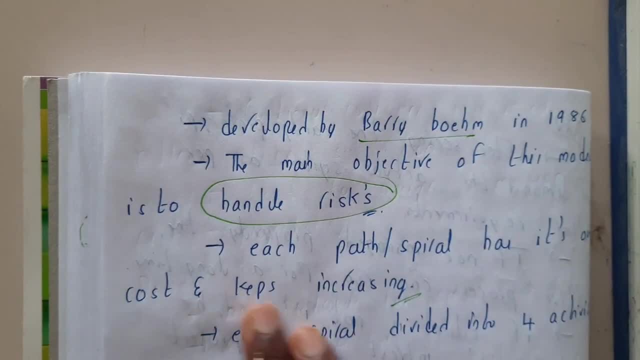 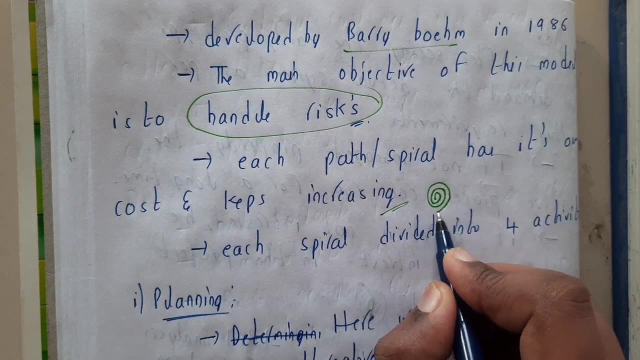 So you can say that it is directly proportional and each spiral has its own cost and it keeps increasing. So you cannot say that the inner spiral is small, so it will be having some least cost It might be, whereas the exterior, as it goes the time and the length of the duration, will increase and the cost will also increase. 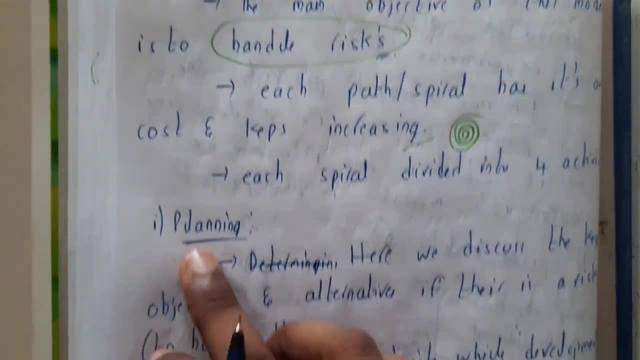 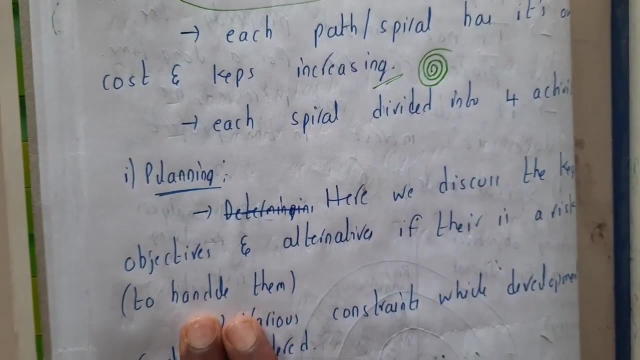 Okay, So each spiral is divided into four steps. that is nothing but planning, So I'll be just giving you a small introduction. guys, Here we discuss the key objectives and alternatives if there is a risk to handle them, So various constraints while developing the project are also considered. 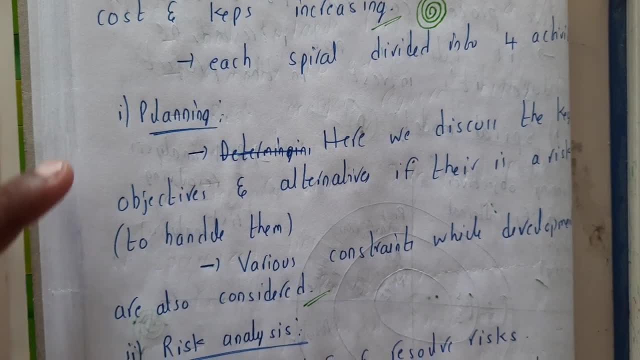 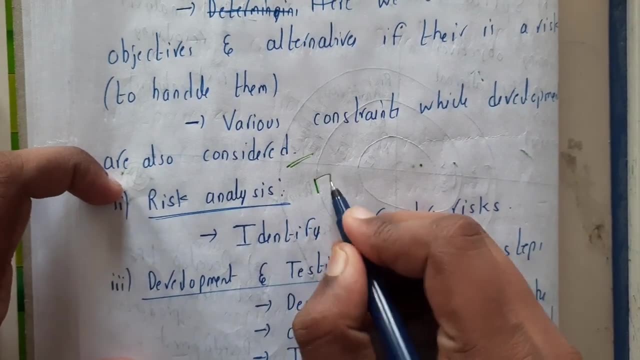 So, basically, here you will be planning, you'll be gathering the requirements and you'll be doing the planning. work guys here. Similarly, risk analysis. So here you'll be identifying the risk and you'll be resolving the risk. So, if there is a risk, what will be the cause for it and what are the issues you'll be getting? 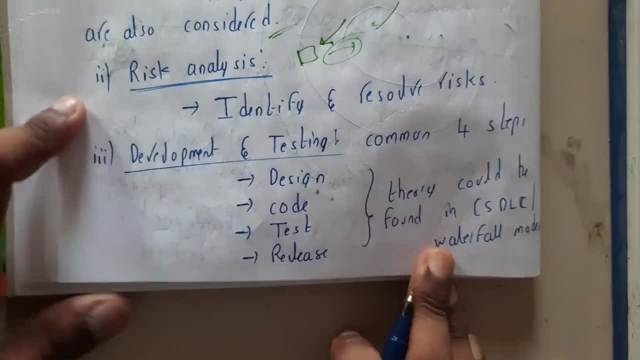 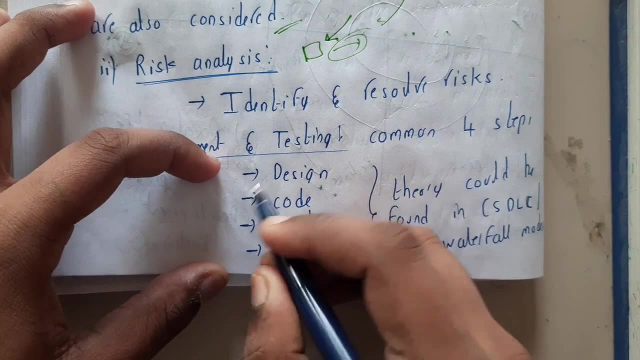 How to resolve it, All those things we'll be discussing here, And the next step is nothing but development and testing. So, basically, here we'll be doing the four basic steps- Sorry, the four common steps- that we are discussing from the start of this unit. 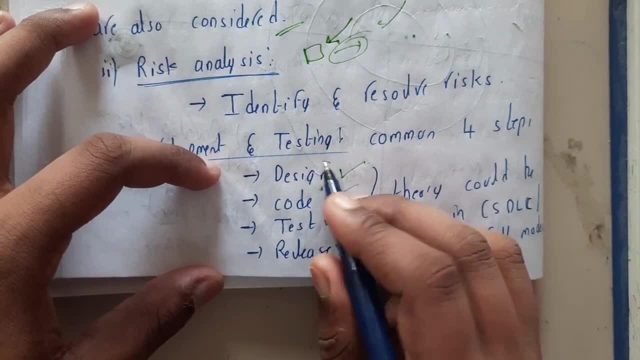 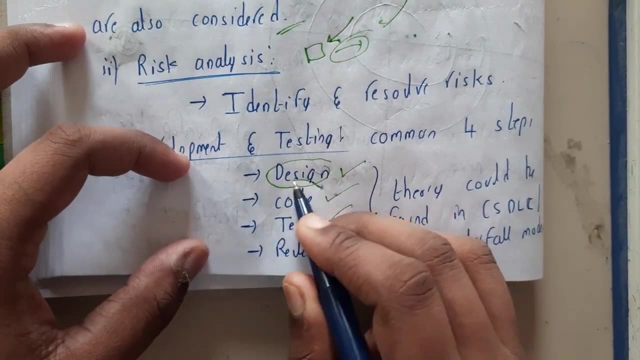 That is nothing but designing, coding, testing and release. So design is nothing but based on your input, the requirements. you'll be designing a particular model. You'll be designing one or two models and among them you'll be selecting one at the end according to the client requirements. 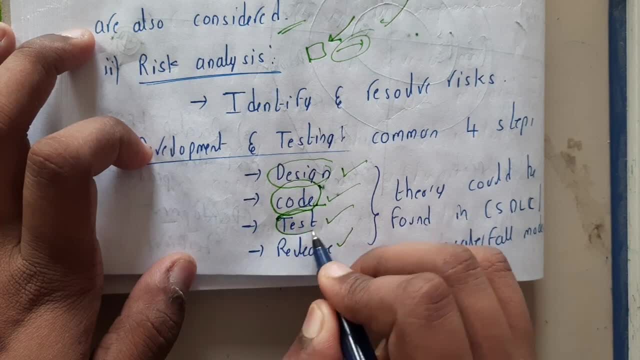 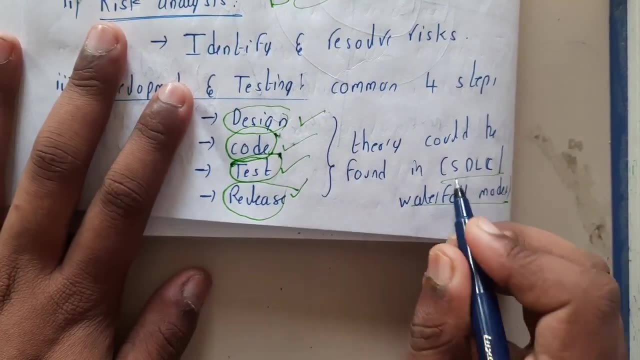 Coding. So you'll be performing the coding based on the design, and then you'll be testing each and every model and integrating them, and again testing. At the end you'll be releasing the product. Guys, you can find the theory for these topics in SDLC or in waterfall model. 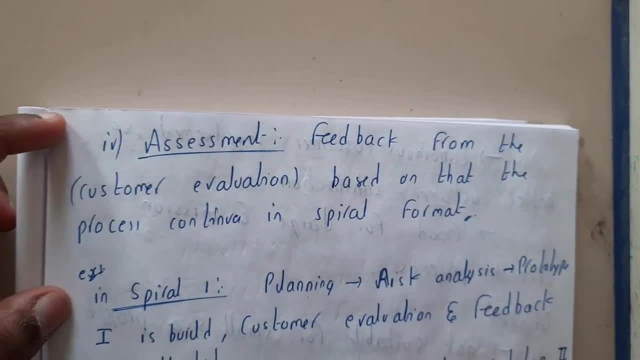 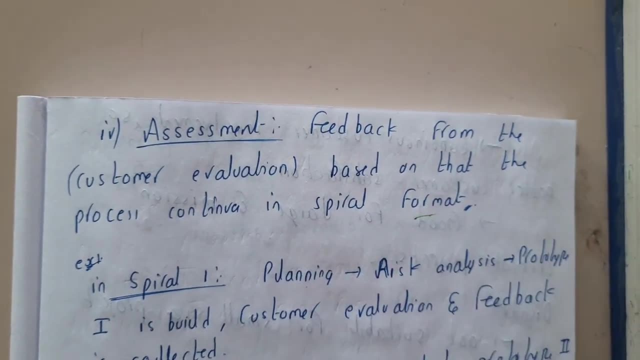 Okay, Okay. Similarly, the last step is nothing but assessment. So, based on the customer feedback, feedback from the customers are evaluated based on the process continued in the spiral format: Okay, Okay. So in our example, we are having three spirals, right? 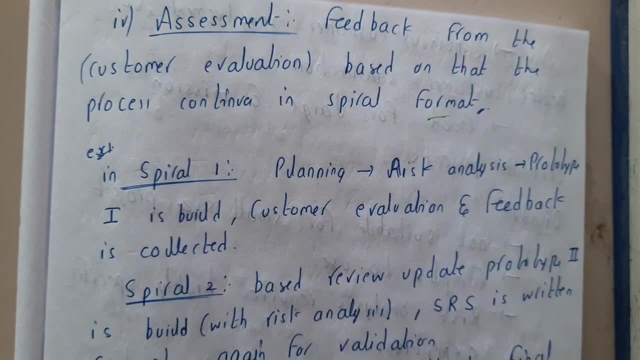 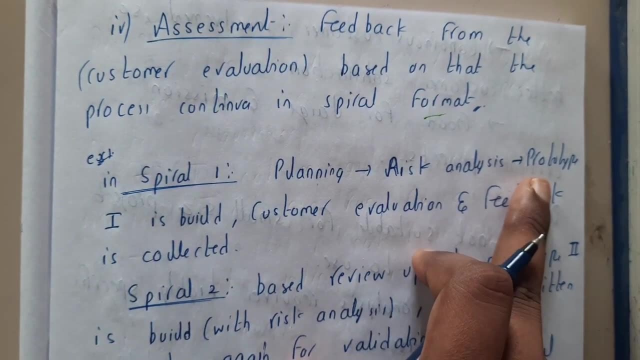 So if we are following three spirals, these are the three spirals, which indicates guys: Okay. So initially, in spiral one, we will be planning, we'll be doing risk analysis and we'll be making a prototype. One is built, Customer evaluation and feedback is correct. 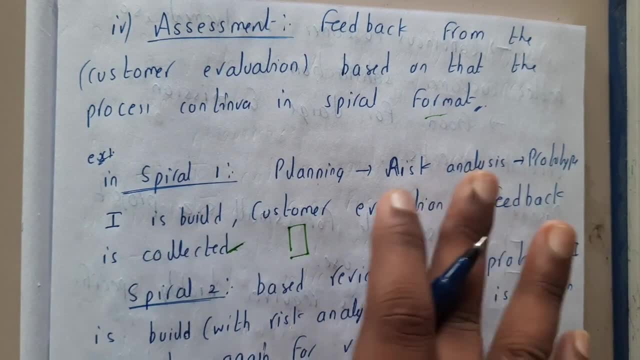 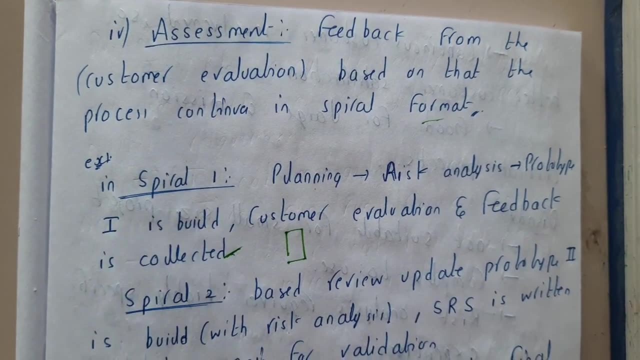 So basically, here in this first spiral, you will not be getting any product like incremental model. You'll be getting one whole process of the spiral is done. In the last stage of spiral you will be starting your development and everything is okay. So in spiral two, based on the reviews provided by spiral one, you will be designing the prototype two. 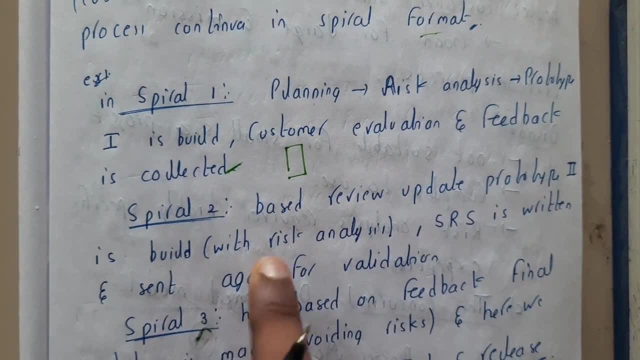 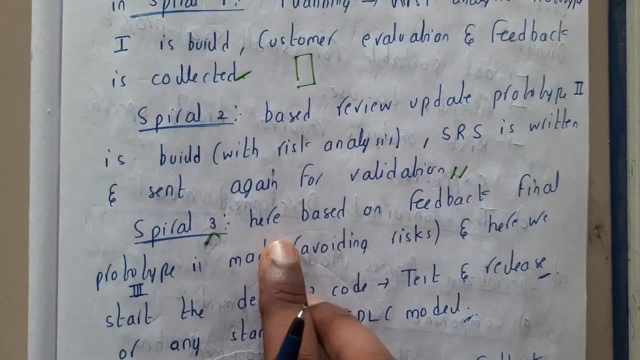 In each and every step you will be calculating risk, guys. Remember, the prototype is built with risk analysis. SRS is a return and send it for evaluation or validation. So once the validation of SRS is done, here you'll be taking the final feedback. 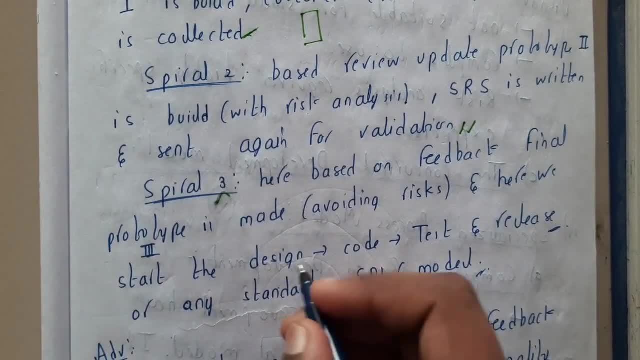 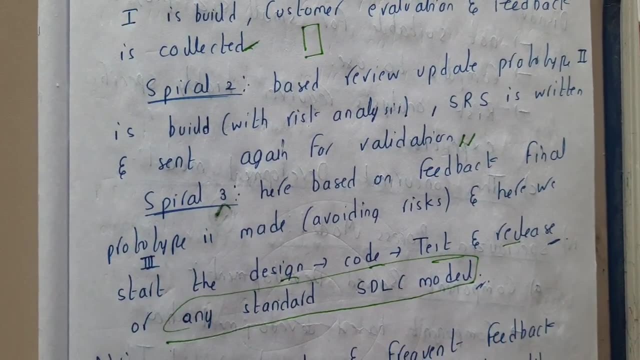 from the prototype and here you will be starting your main process, guys. You'll start design, coding, then testing, then release or if any other things which are required in SDLC- everything you can do it here, right? Yes, So I hope everyone got a small idea on spiral model. 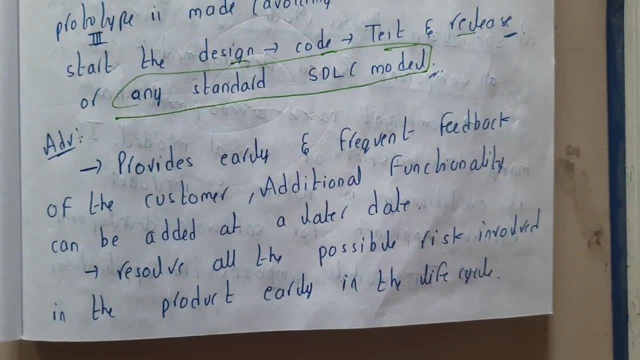 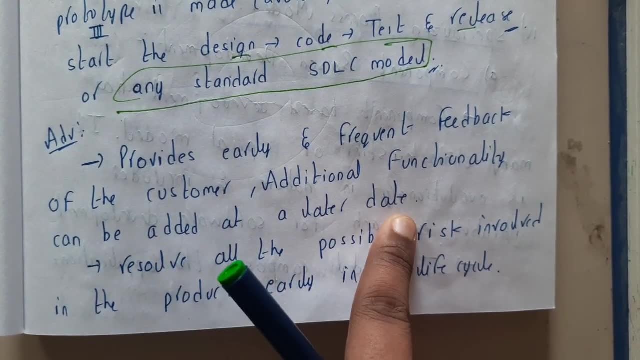 So let us continue with some advantages and disadvantages. So the main advantage in spiral model is that it provides early and frequent feedback of the customers. Additional functionalities can be added at later date also, So additional functionalities can be added any time you want And the customer feedback is the first priority right. 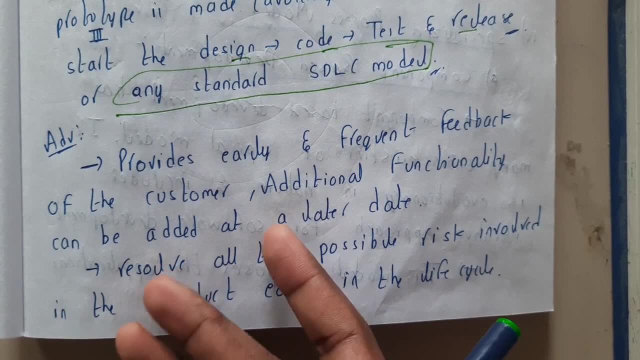 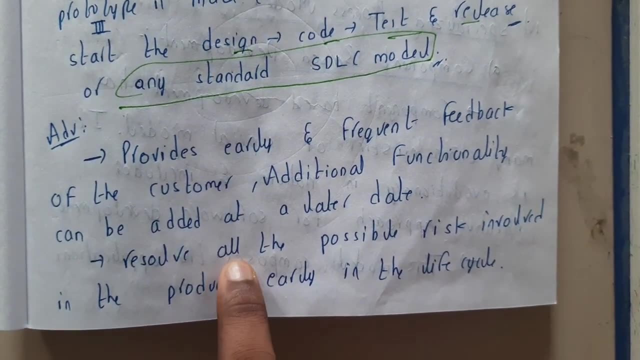 So you are designing the product for the customer. So if the customer is not satisfied, what is the use of your product then? right, That is the reason why the customer satisfaction is really important. Then resolve all the possible risks involving the product: early life cycle. 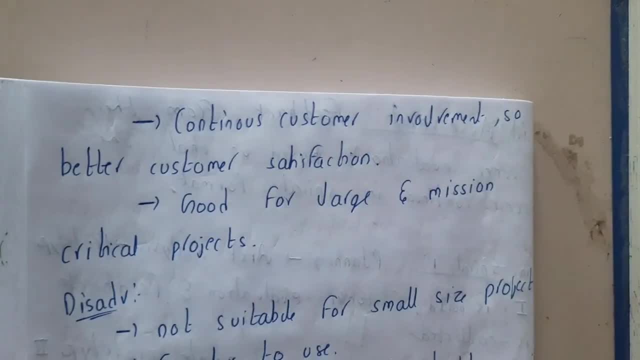 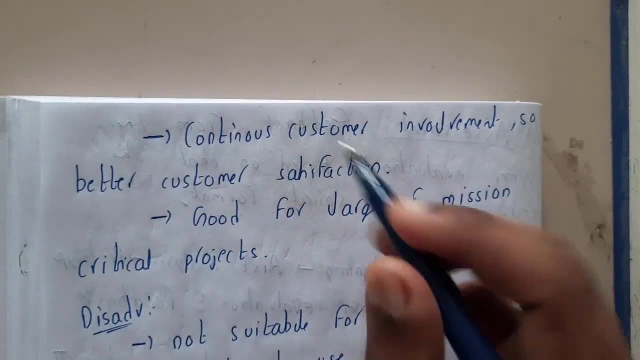 So basically you are doing risk analysis right. So that is the reason why the risk analysis is done, So there will be no further risks in releasing the product or anything. So continuous customer involvement is there, So customer satisfaction will be high. good for large and machine and machine critical projects. 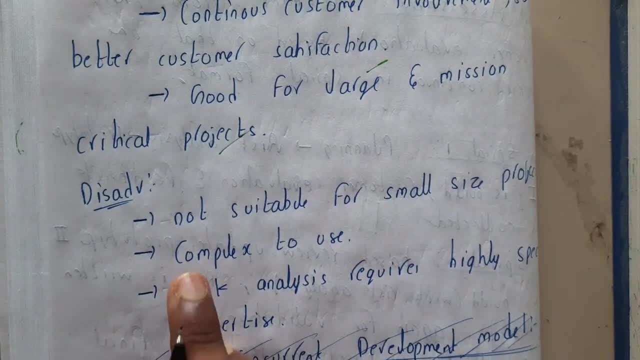 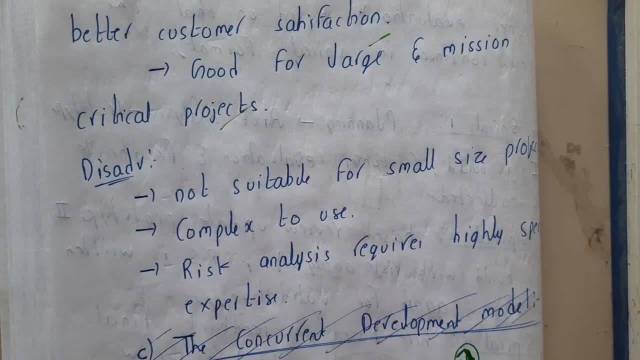 So basically for large projects we'll be using this kind of approaches. So disadvantage, So not suitable for small projects and complex to use. So basically risk analysis and everything will be a bit complex when compared to normal guys. Yeah, that's what it's written here.